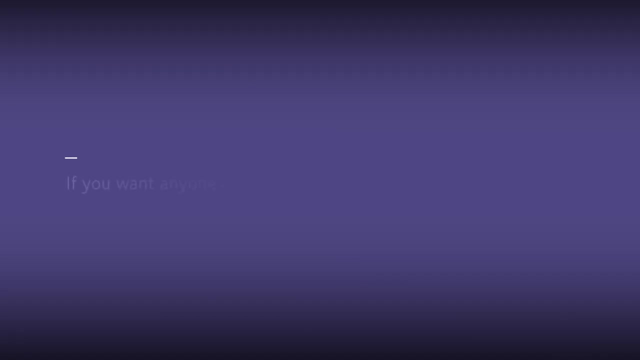 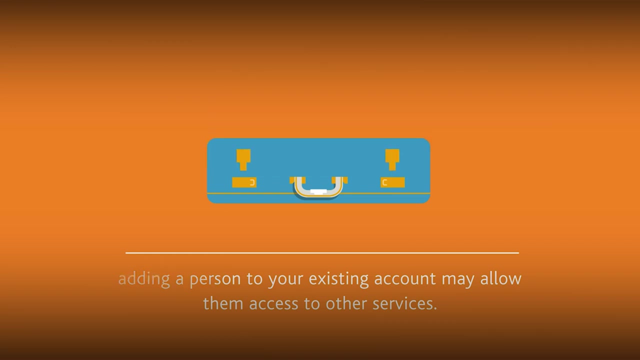 other Government Gateway services. If you want anyone else to use the service on your behalf, it's advisable to create a new account. Adding a person to your existing account may allow them to access other services. You can choose to create either an individual or organisation account. Select the individual. 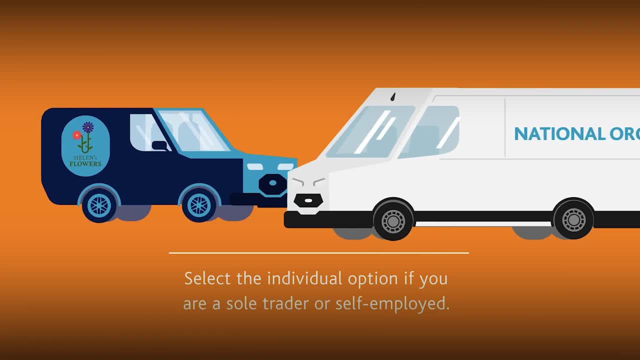 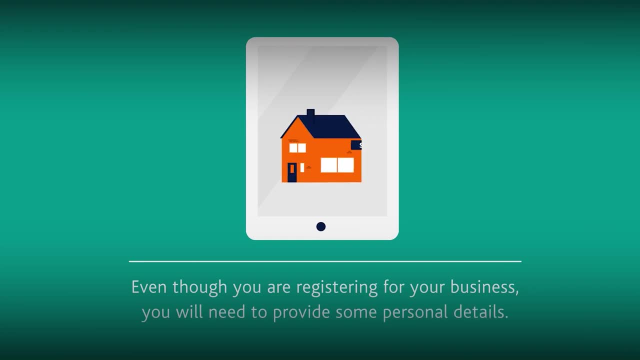 option if you are a sole trader or self-employed. If you need to add anyone else, you'll need an organisation account To register for your business, you will need to provide some personal details Apart from the contact information. the Valuation Office Agency does not retain or use this information. 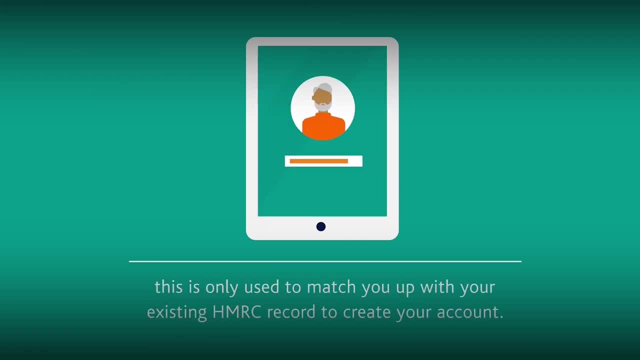 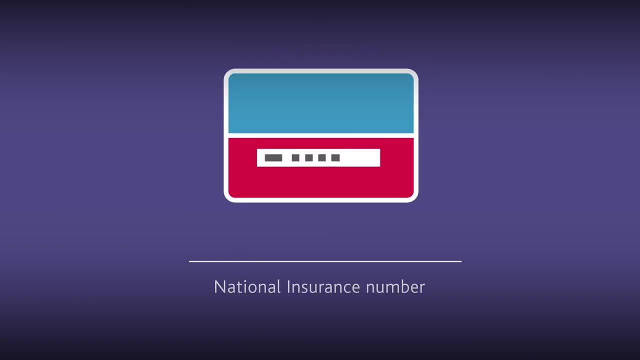 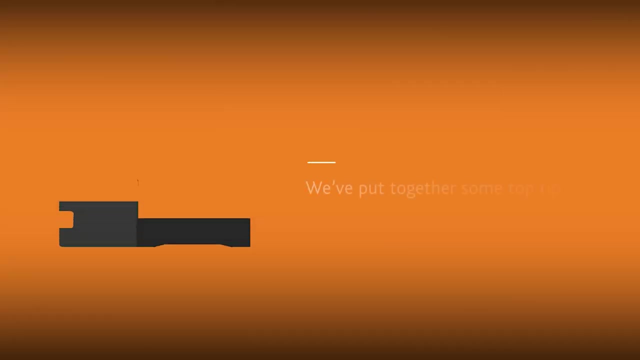 It is only used to match you up with your existing HMRC record. to create your account, To register, you need your date of birth, national insurance number, details from at least one of either a payslip UK passport or P60.. We've put together some top tips to 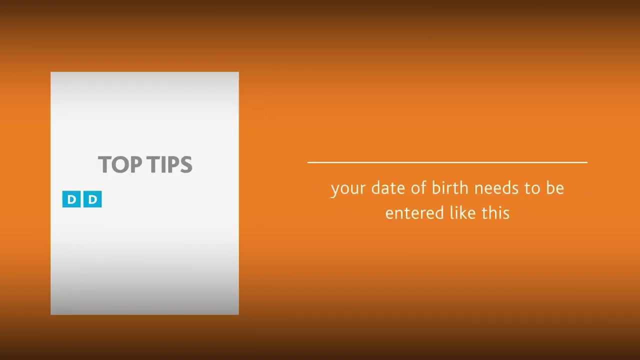 make this process easier, Your date of birth needs to be entered like this: Date, month, year, eg 21-04-1985 or 7-12-1978.. The letters in your national insurance number should be in capitals. Your first and. 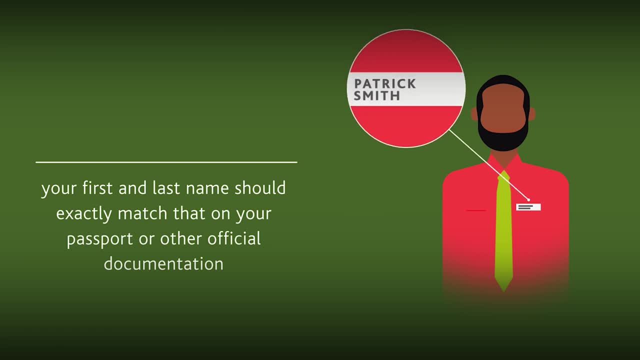 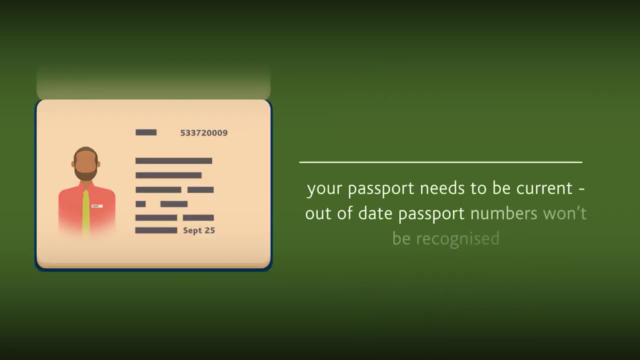 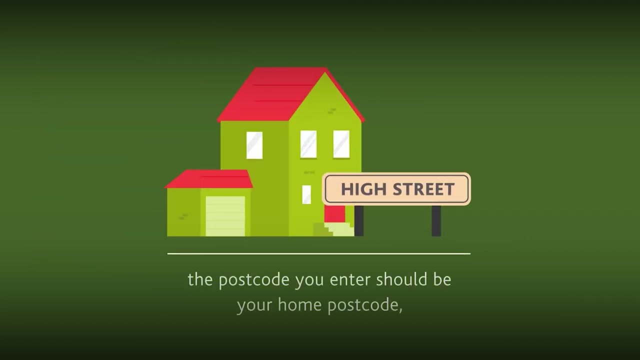 last name should exactly match that on your passport or other official Government documentation. Otherwise we won't be able to find your address. Your passport needs to be current. Out-of-date passport numbers won't be recognised. The postcode you enter should be your home postcode, because that's what HMRC holds. 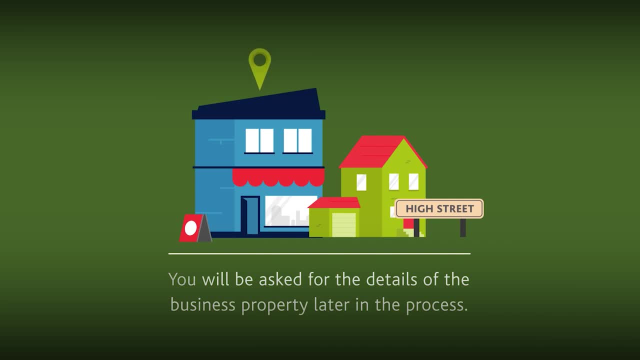 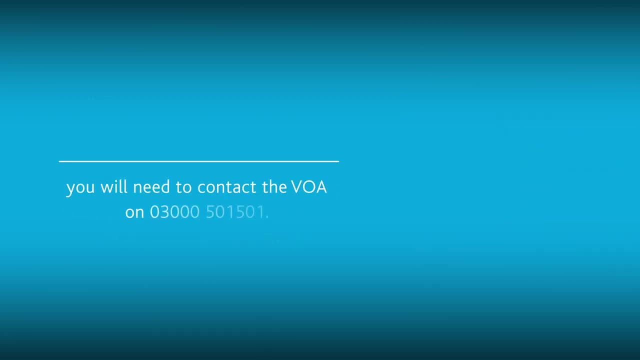 You will be asked for the details of the business property later in the process. If you are self-employed and do not hold a UK passport, or if you are still having trouble registering, you will need to contact the Valuation Office Agency on 03000.. To register, you will need to contact the Valuation Office Agency on 03000.. To register, you will need to contact the Valuation Office Agency on 03000.. To register, you will need to contact the Valuation Office Agency on 03000.. 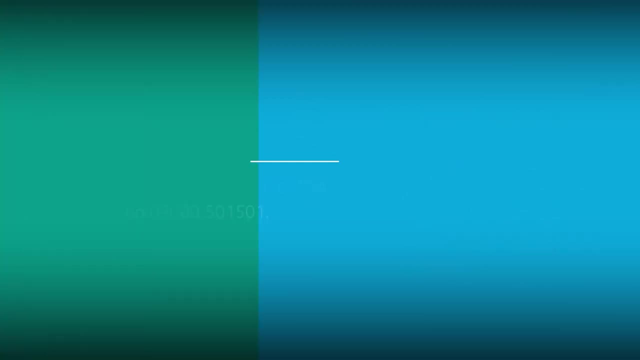 Once you have registered, you can claim the property or properties that you or your business are connected to. You will then be able to see or request the detailed property information.